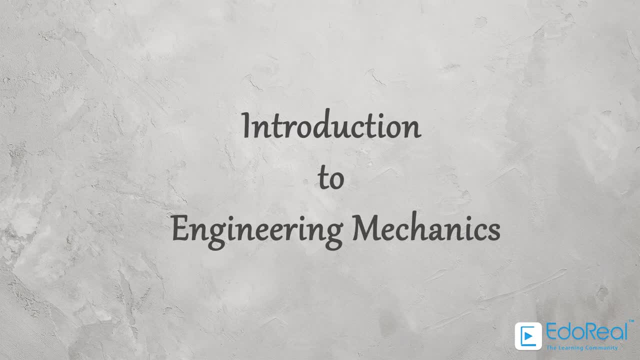 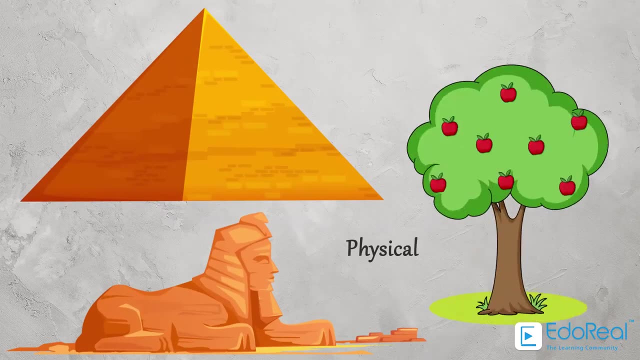 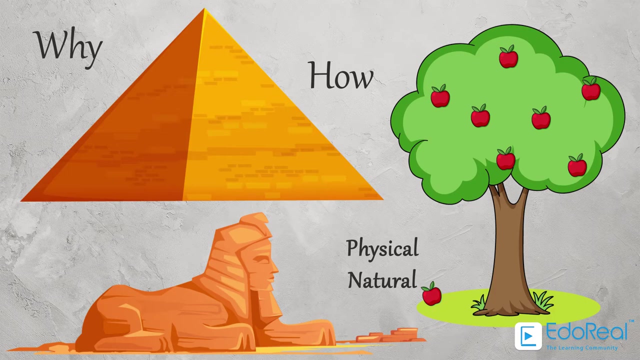 In this video we will discuss about introduction to engineering mechanics. We cannot learn engineering just by reading books. We have to look at physical systems as well as natural systems around us and ask questions such as why and how these are made the way they are. Let's imagine driving a bike on a wet road As the force of friction which 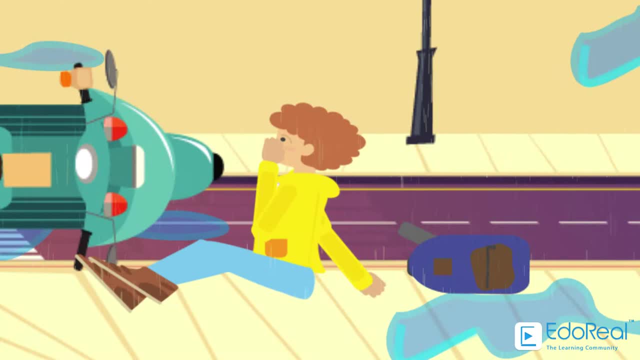 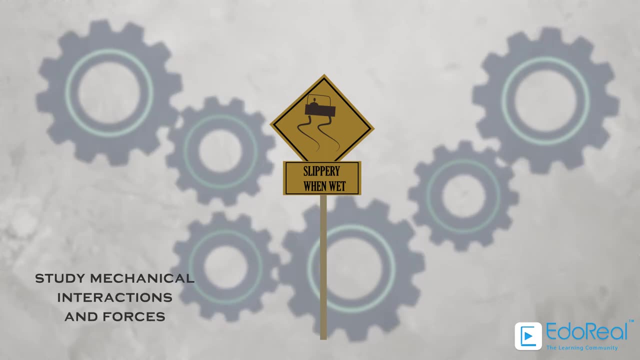 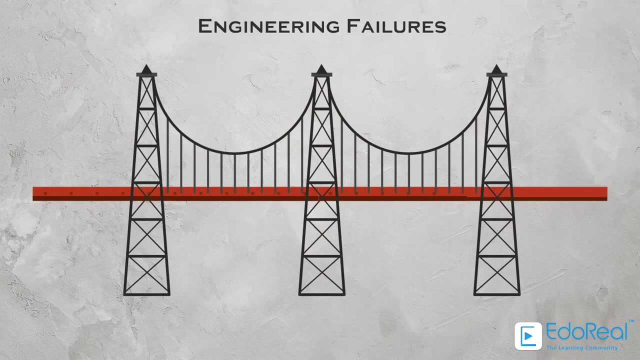 holds, the bike will be low. on wet roads we may fall down. So it is better if we study mechanical interactions between different bodies and effect of forces acting on them, so that we can avoid such mishaps. We have seen the failure of many structures like bridges. 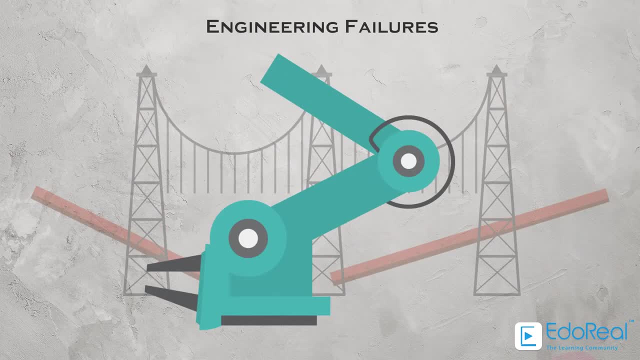 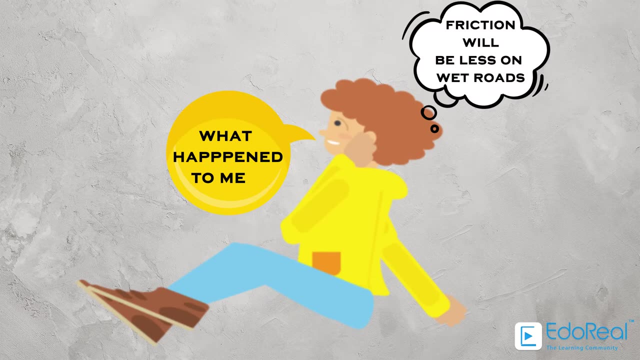 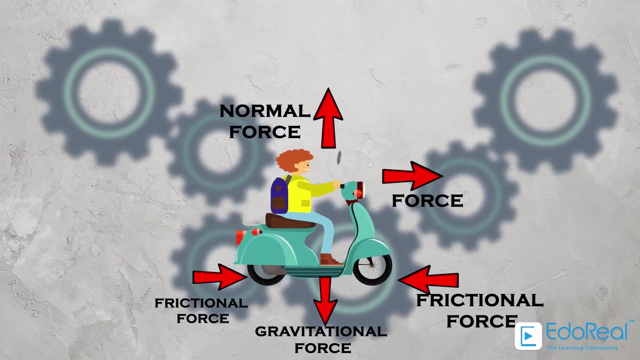 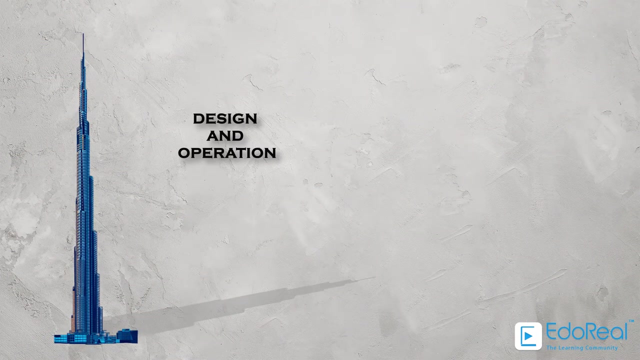 rockets machines because of engineering failures that happened majorly due to neglecting forces acting on them. We can learn so much from failure than success. If we can thoroughly understand all the forces acting on a system, we can create engineering wonders. Burj Khalifa in UAE is the tallest living structure. 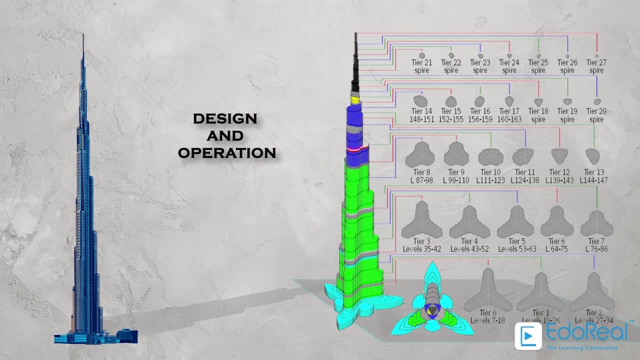 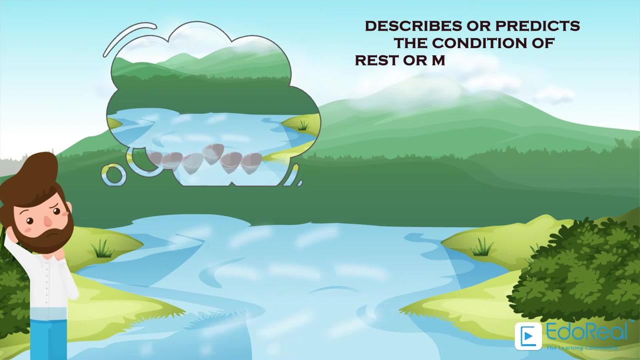 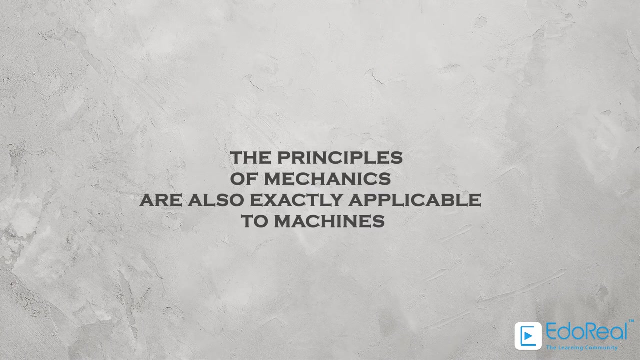 till now, From its foundation to its structural components and mechanical systems. The design and operation of the tower is based on the fundamentals of engineering mechanics. Mechanics is the science. Mechanics is the science which describes and predicts the condition of rest or motion of bodies under the action of forces. The principles of mechanics are also applicable to machines. 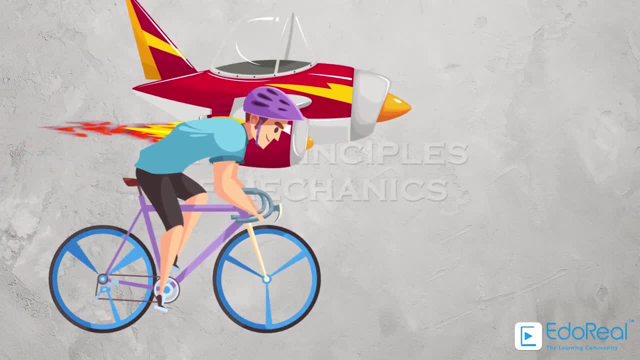 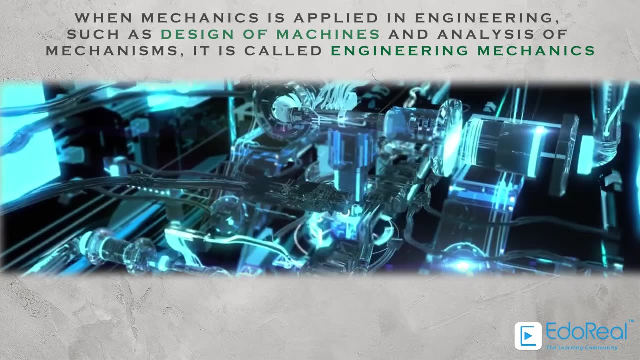 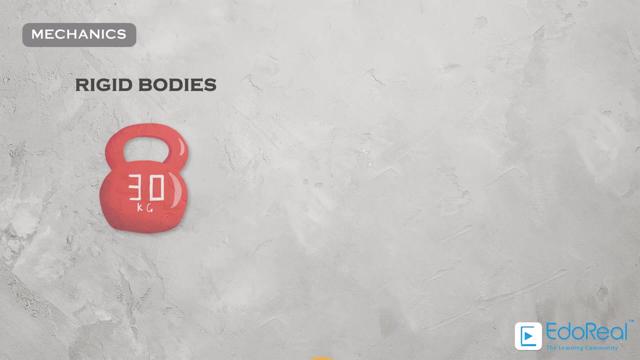 It may be a simple machine such as a bicycle, or a machine as complex as an aircraft. When mechanics is applied in engineering, such as design of machines and analysis of mechanisms, is called engineering mechanics. It consists of the mechanics of rigid bodies, mechanics of 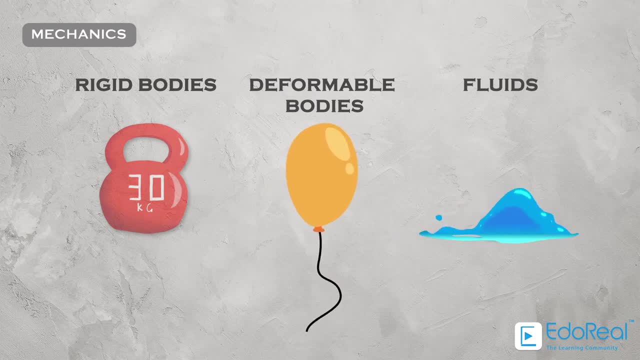 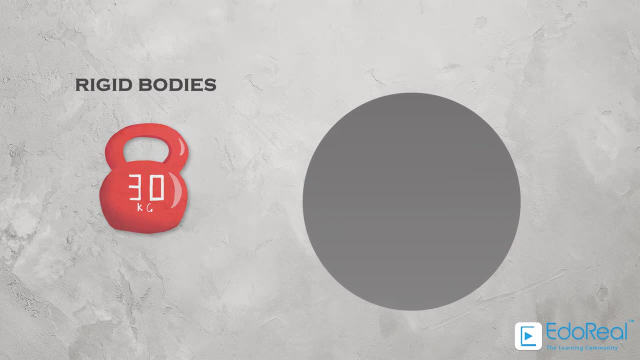 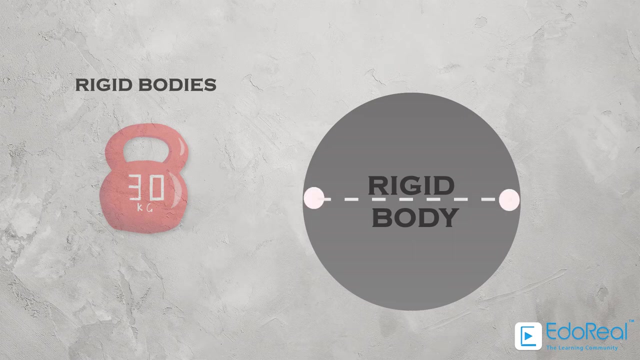 formable bodies and mechanics of fluids. In this subject we are mostly concerned with the mechanics of rigid bodies. Let's see what is a rigid body first. Rigid body: A body is formally regarded as rigid if the distance between any set of two points in 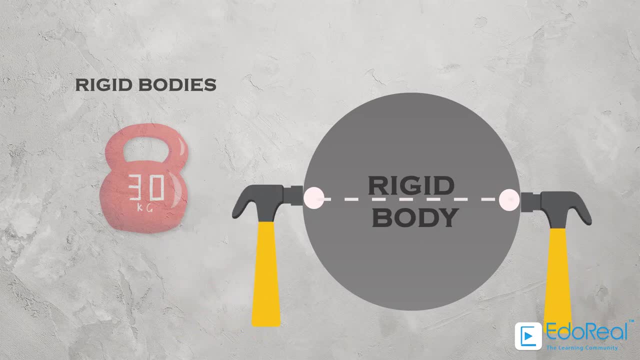 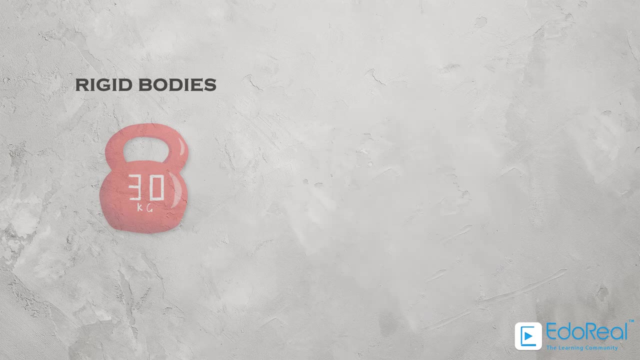 it is always constant in time, regardless of external forces exerted on it. This basically means that you can't deform it by any means. It's somewhat an indestructible thing. The closest you can get to a rigid body might be diamond, carbon nanotubes or its derivatives. In real life all.